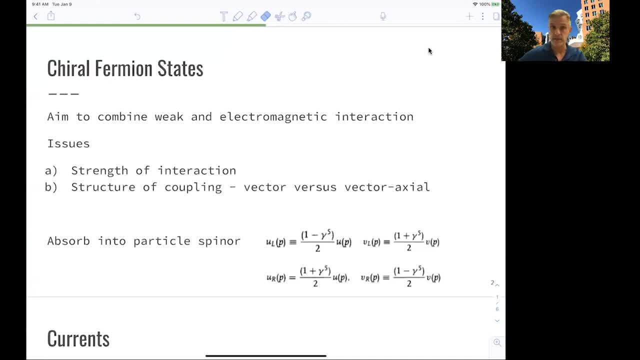 This one minus gamma five, This vector minus axial coupling. So one way to mitigate this problem is to simply absorb this one minus gamma five term in the definition of the particle spinors And I have to warn you this is a little misleading and I think that led also to some of the confusion we had in the class before. 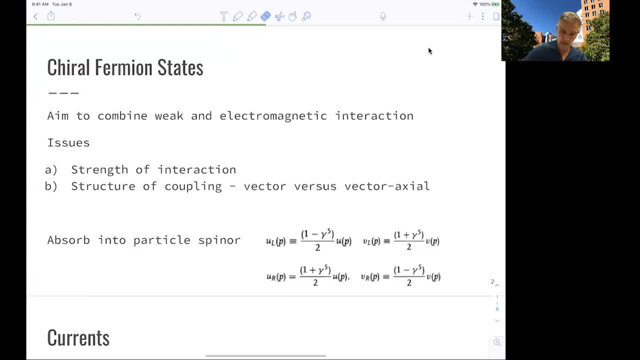 So what we're doing here simply is we take our spinor and we project out with a one minus gamma five term what the left-handed component of this spinor is. This is just a projection and the definition of this, and we can do this for antiparticles as well as for the right-handed components as well. 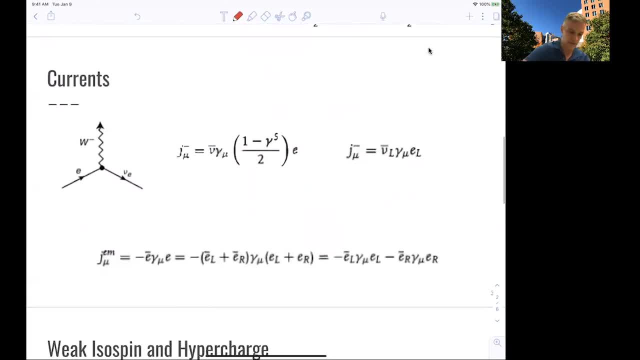 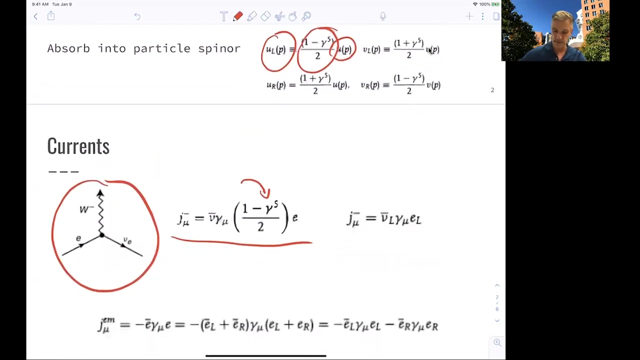 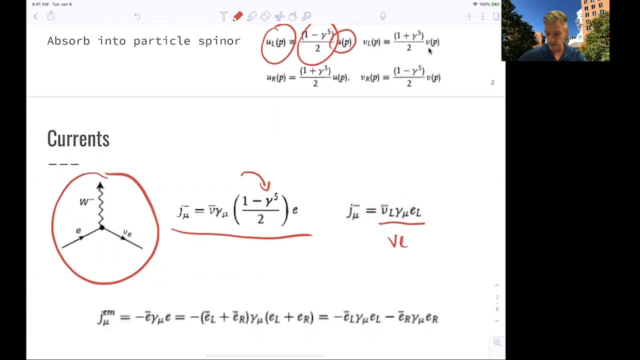 Good. So now we can look at the currents again and we look at this weak current, What we have seen. we can write, as you know, our antineutrino here, gamma mu times one minus gamma five half. Now, if we now define our particles with gamma matrices, we find that, oh, this simplifies quite a bit because we now find the current which can be simply written as a vector current. 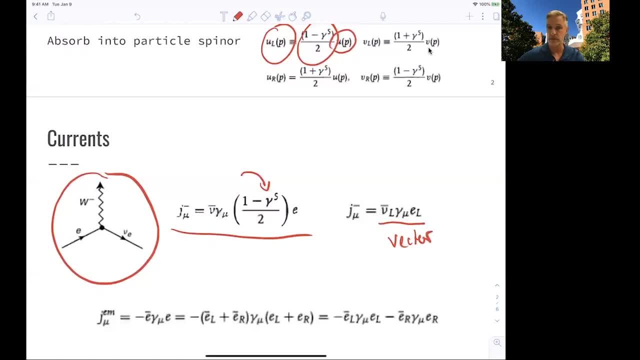 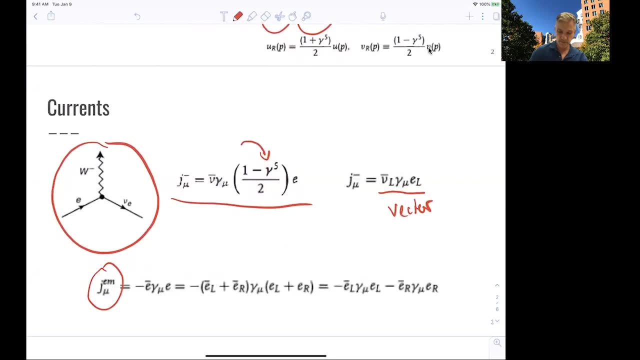 So we mitigated this quite nicely. So what now happens to our electromagnetic interaction here? So we have an electron coupling to a photon, We can project out the right-handed and left-handed component, and then we have to add them together again. 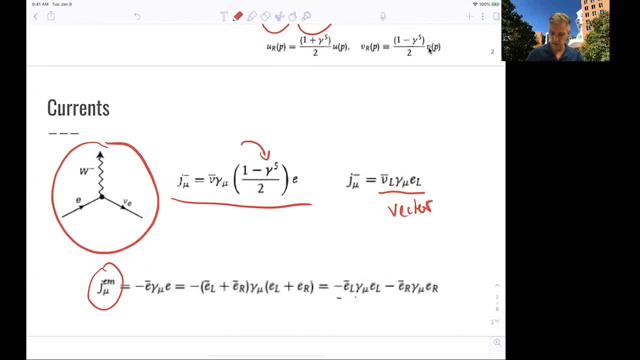 When we do this, we find that, huh, there is a component of the left-handed component, a current corresponding to the left-handed particle and the current corresponding to the right-handed particle. There's no mixed term here because of the way gamma matrices, or gamma five matrices, multiply. 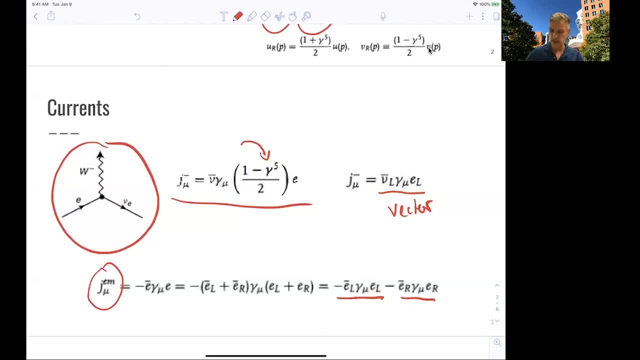 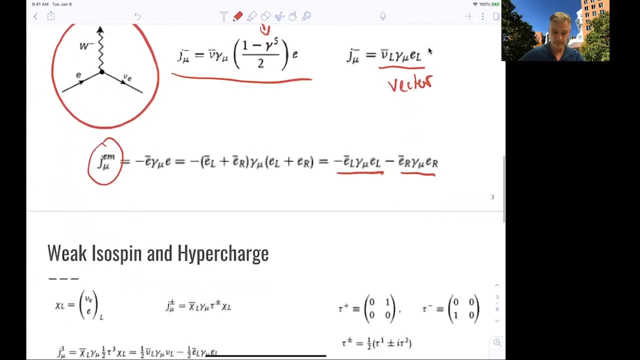 So that's nice. This also explains why the helicity is not changed in QED. We basically see this from the algebra involved in those equations. Good, So far we haven't done anything. We have just changed the notation. 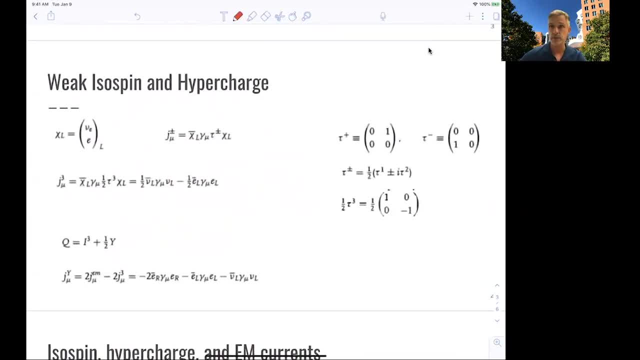 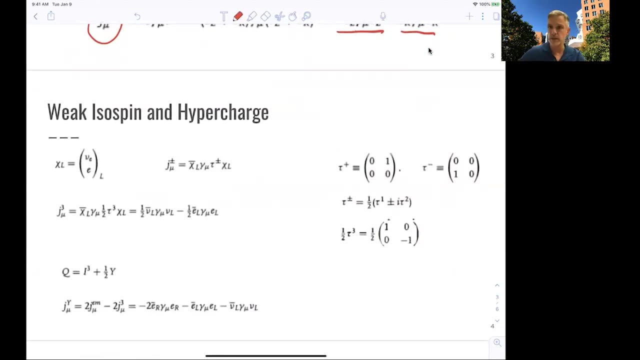 So we can go one step further and reuse the concept we introduced when we talked about QCD or the strong isospin, And, since we can nicely describe those currents here of those particles, maybe see if we can write an neutrino and an electron as part of a duplet. 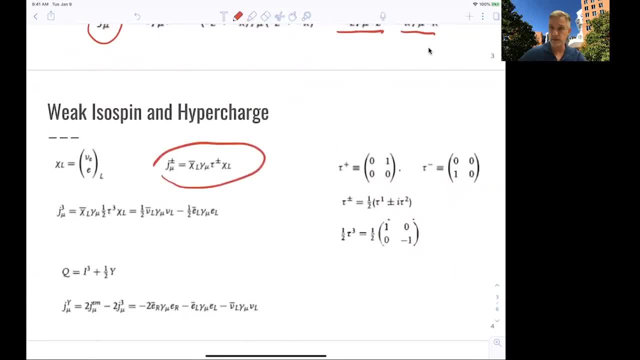 And when we do this, we rewrite the currents, the positively charged and the negatively charged current, as simply the left-handed components of those duplets. We introduced a new matrix here, tau plus and tau minus, and they're simply combinations of tau one and tau two. 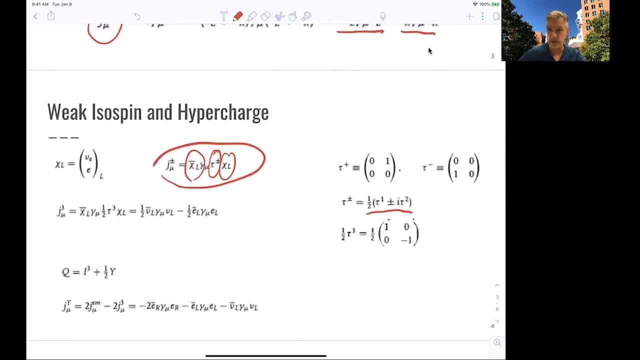 which are in fact the Pauli matrices. It's just a relabeling as well. So there's a lot of relabeling going on. not to confuse you, but we have simply written this current, this positively charged weak current and negatively charged current. 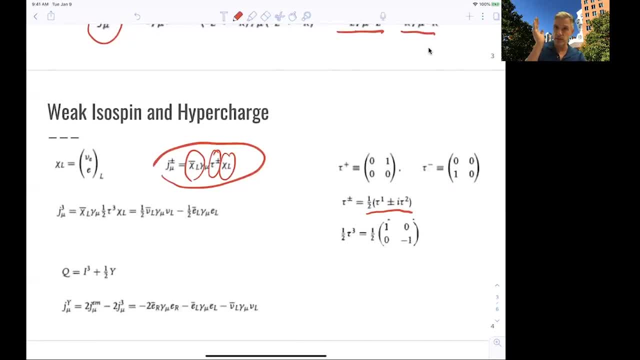 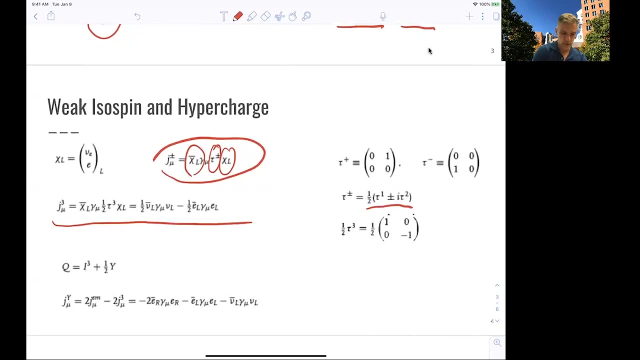 where we rotate a neutrino into an electron or an electron into a neutrino using the weak interaction. Great. So now we can write this current here as a third component of this current. And we see when we write down the third component of this current using tau three here: 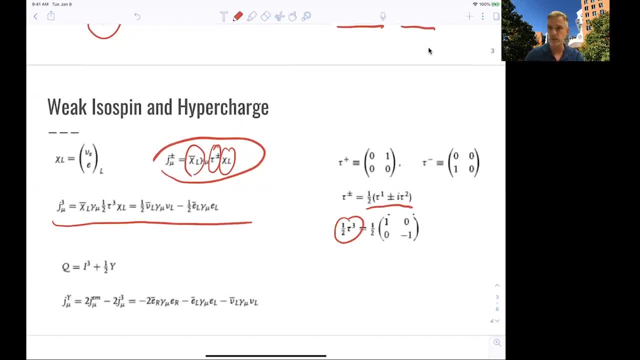 we find that something looks, something which looks like a neutral current right. So this is something like a neutral current, where we have a neutrino coupling to a neutrino and the left-handed electron coupling to a left-handed electron by a vertex vector. 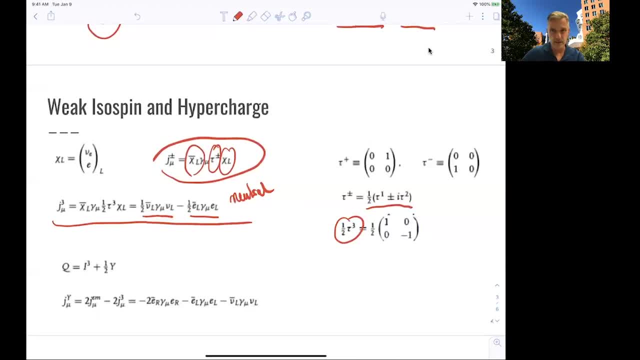 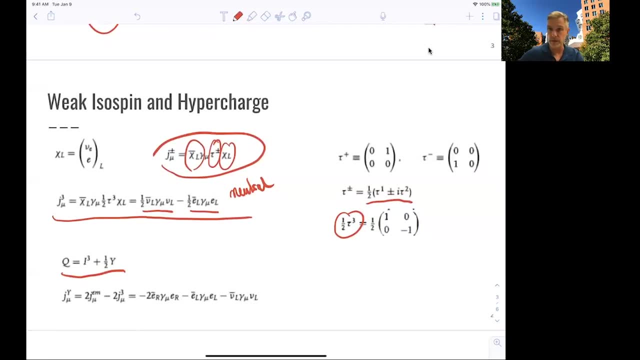 where there's an interaction with those going on. This is not quite the full story yet. Let me remind you about the definition we used also in isospin, which is the Gelman-Nishijima equation, which connected the electric charge to the isospin in the strangeness of the particle. 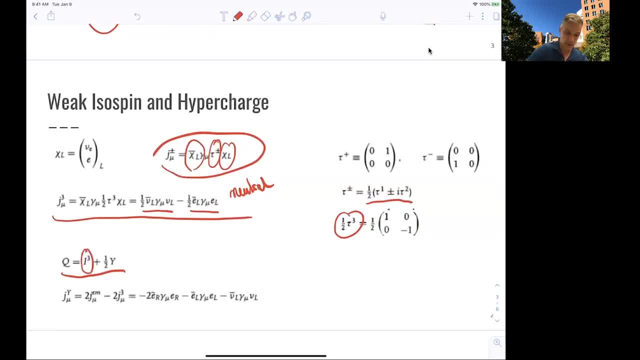 And we do the very same thing. We have an isospin component and a so-called hypercharge component- It's similar to the strangeness we had before- And Q is the electric charge of the particle involved, And so with this, we can now define an isospin, a hyperspin current. 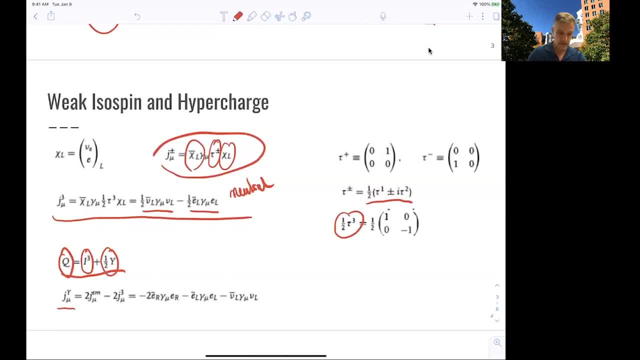 which is given as two times the electromagnetic current minus two times the third component of the V current here And so now we find interesting effects here. So there's a new component which also couples the right-handed particles, So the missing part here. some might have seen this already. 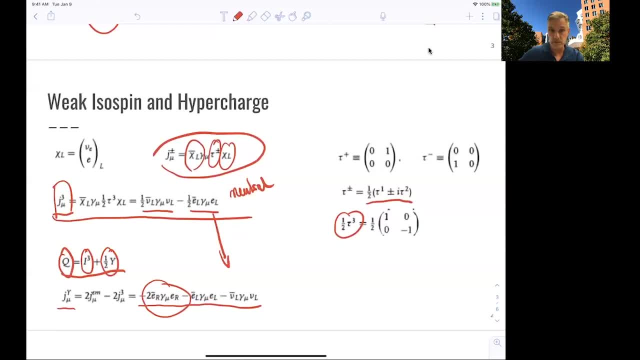 that this neutral current in the upper equation didn't connect or didn't have a contribution from right-handed particles. And since there's right-handed electrons which couple to Z bosons, there needed to be this kind of additional charge. So now we have a current which includes the right-handed particles as well. 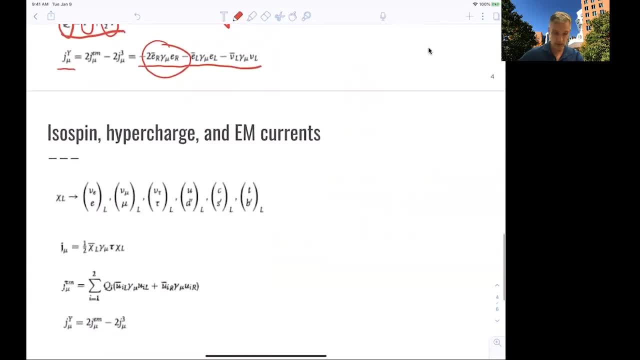 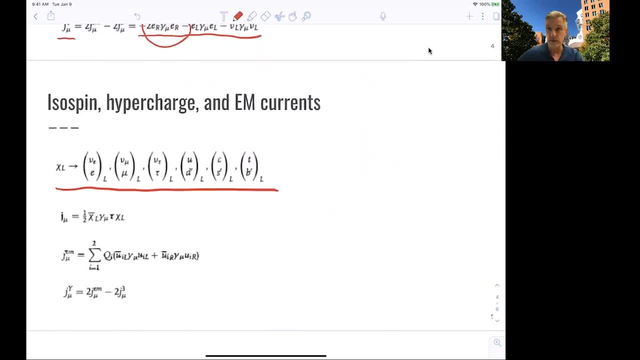 So that's great. We can generalize this by writing those duplets for all particles. we know There's an additional kind of caveat here. We haven't talked about this too much. We have to consider the fact that mass eigenstates are not really the same eigenstates. 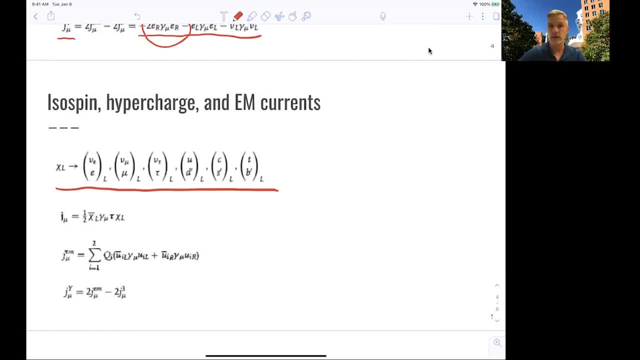 which participate in the weak interaction. Right now we can ignore this. We'll later come back to this question- And then we can write the three components of our isospin current and our hypercharged current as well. Note that this EM current here is our electromagnetic current. 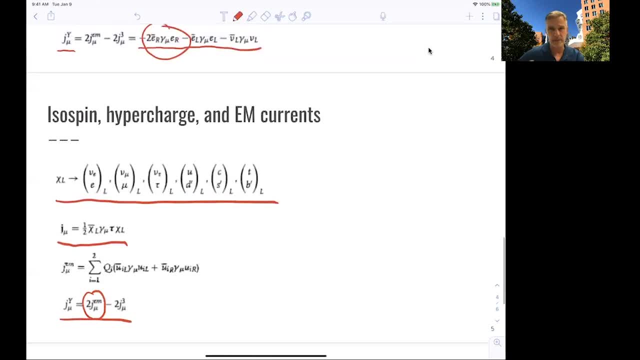 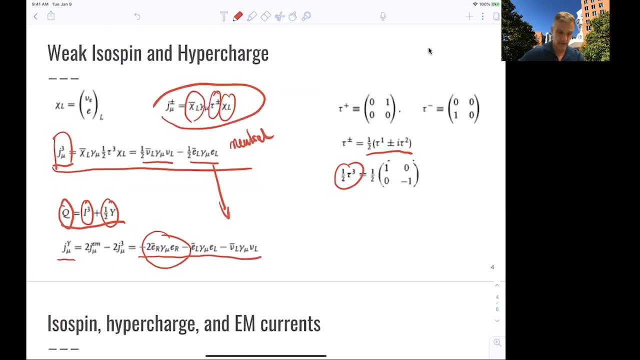 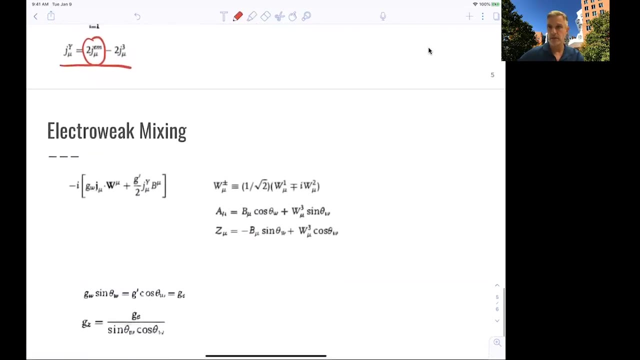 Good. So now we wrote this and we find somehow very close, a consistent picture. We find that there is a charged current and then there is a neutral current in the weak interaction, But what we actually wanted to do is combine the weak interaction and the electromagnetic interactions. 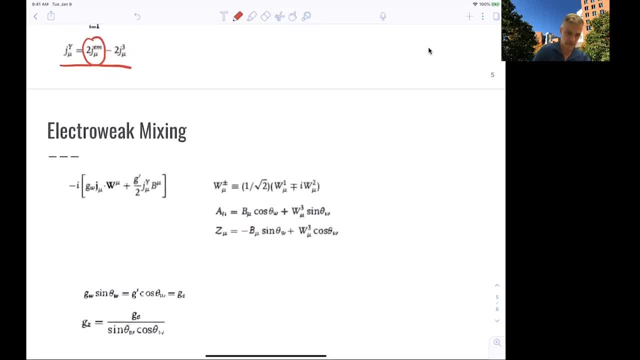 Now let's look at this again and start over again. So we have an isospin current here which couples to the three components, the triplets, the isospin triplet. So this is a W1, W2, W3 triplet. 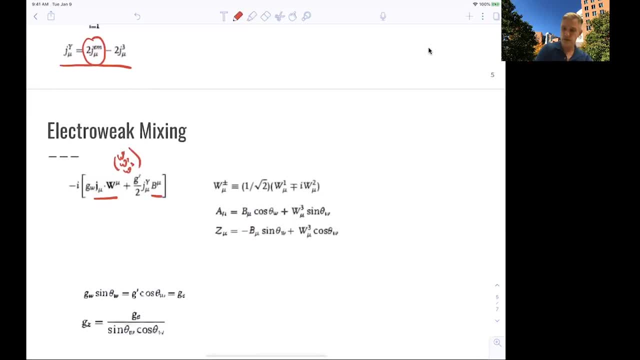 And then we have the singlet here which couples to the hypercharge. Very good. So now, if I try to identify now components which we already know, the first thing we can do we have to make sure that we find our W plus and W minus bosons again.